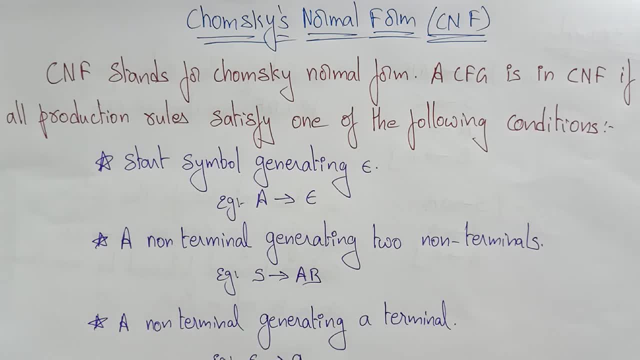 Hi students, welcome back. Coming to the next topic, that is a Chomsky Normal Form, CNF. So far you had seen about the CFG, that is a Context Free Grammar. CFG means Context Free Grammar, whereas CNF is Chomsky Normal Form, So don't be confused. it is FG Whenever you have. 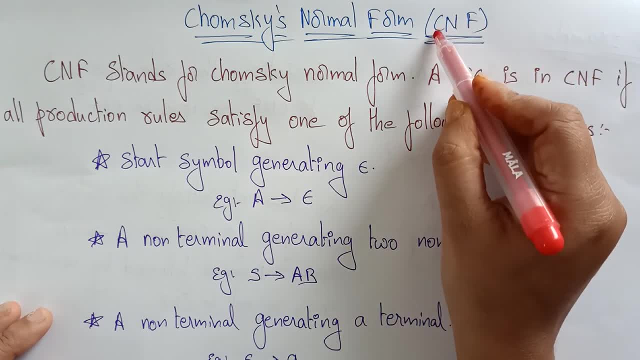 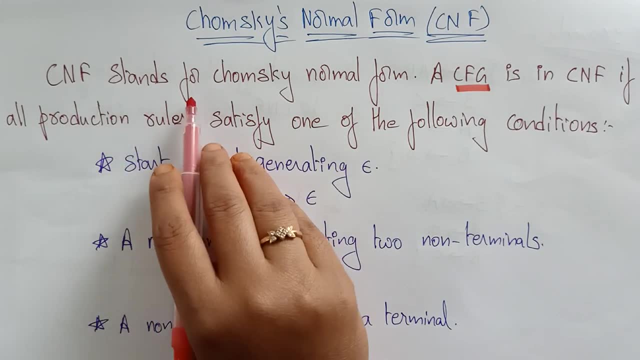 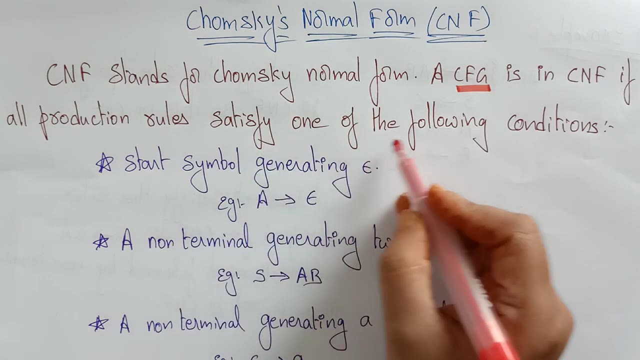 seen this Context Free Grammar: CNF is Chomsky Normal Form. So what is this? Chomsky Normal Form A? CNF stands for Chomsky Normal Form. A Context Free Grammar is in CNF if all production rules satisfies one of the following conditions: When you can say that the given grammar that is a. 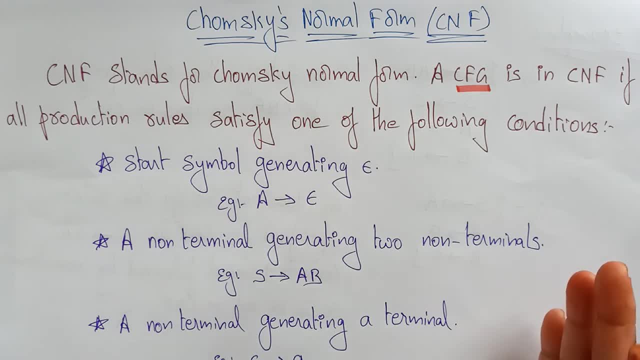 Context Free Grammar is in CNF. If all the production rules are following any one of these conditions, then we can say that the given grammar is in Chomsky Normal Form. Okay, so the production rules, whatever the production rules you are seeing with the starting symbol. 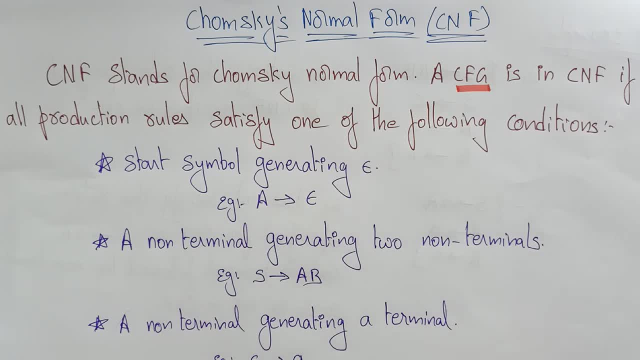 and with non-terminals on the left hand side and the terminals and the non-terminals that are present on the right hand side, that productions. you call it as a Context Free Grammar That we know that. So all the production rules are in the form of Context Free Grammar. If you want to find 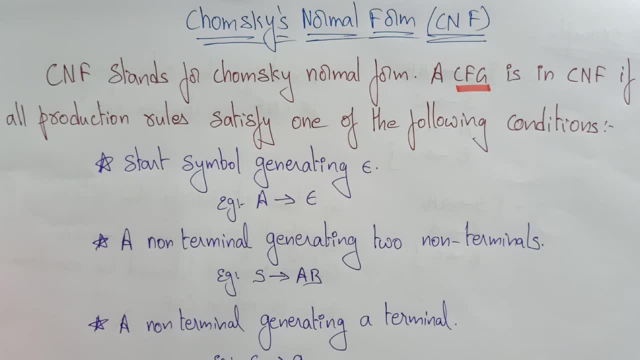 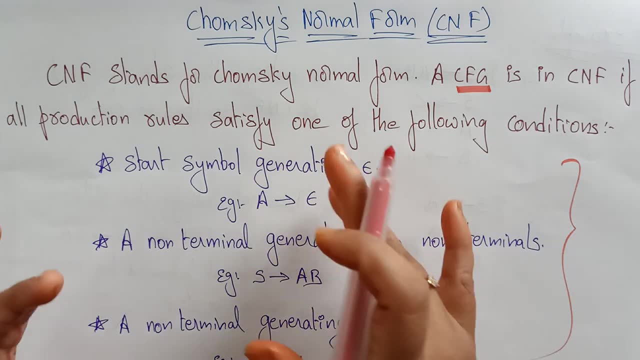 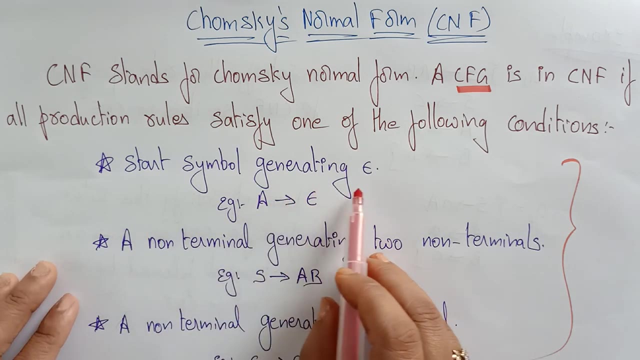 out whether the given Context, Free Grammar, is in the Chomsky Normal Form or not. these conditions has to be followed. Anyone has to be satisfied. Okay, any one of these conditions has to be satisfied In the given production rules. what are those conditions? The start symbol generating Epsilon? okay, the start symbol. whatever the 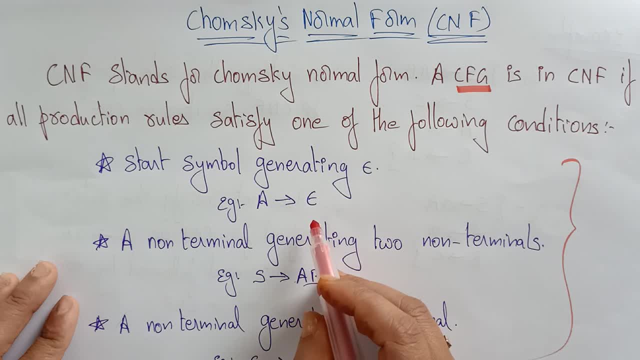 symbol that is starting with that the start symbol is generating is Epsilon, Then you can say that the given Context- Free Grammar, is in Chomsky Normal Form or a non-terminal is generating two non- terminals. so if the grammar is in the form of like this: n sagt: fik ssik. a non-terminal is generating two non-terminals. Stan inspirasil dirkomerenu engluan amby kranjak. a non-terminal is generating two charmals. a non-terminal is generating two charmals. so if the grammar is in the form of like this: n sek Chinaiter klas encontra klasik. 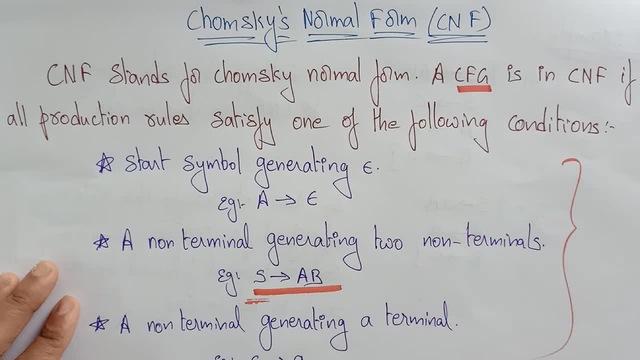 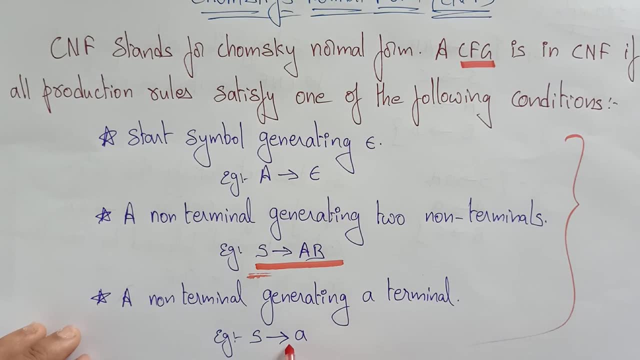 two non-terminals, then you can say that the given grammar is context-free grammar is in Chomsky normal form and the third one, or a non-terminal, is generating a terminal, then you can say that the given grammar is in Chomsky normal form. I hope you understand. what are the conditions that? 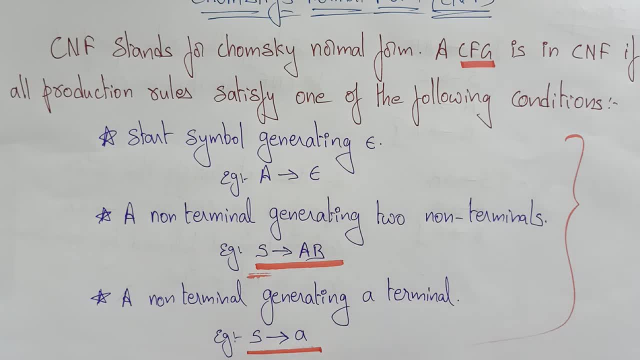 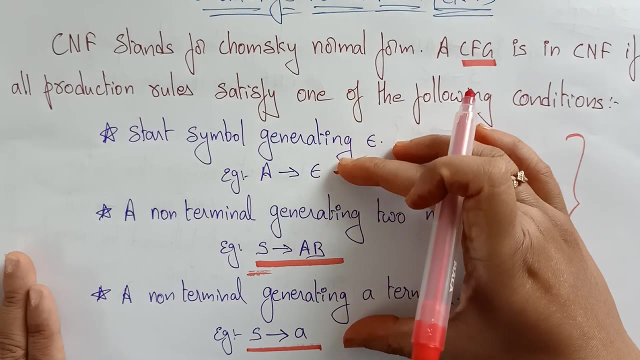 has to follow whether the given grammar is in Chomsky normal form. The conditions are: the star symbol is generating the epsilon or the non-terminal is generating two non-terminals or the non-terminal is generating a terminal. then you can say that the grammar is in Chomsky normal form. So remember. 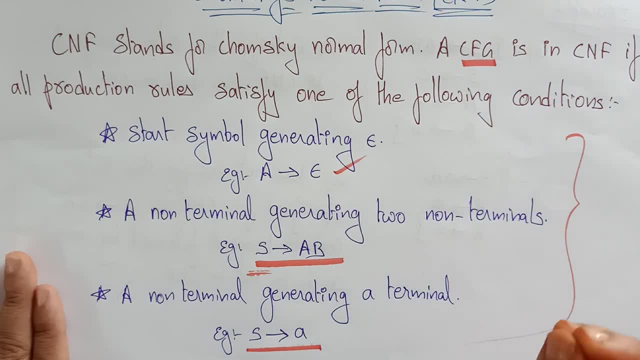 these points. whenever you are seeing the predictions, you can clearly understand. you have to identify not only the understand, you have to identify whether the given grammar is in Chomsky normal form or not. How can you identify? By following these rules. a star symbol should start with an. 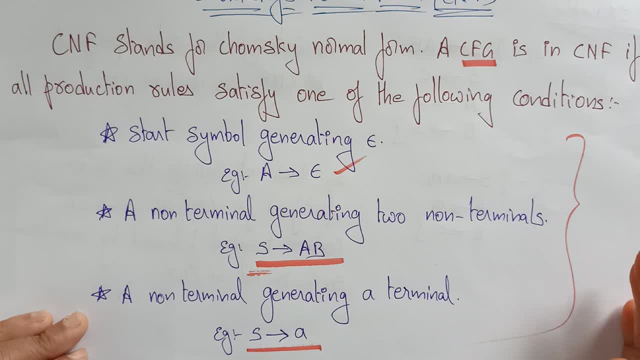 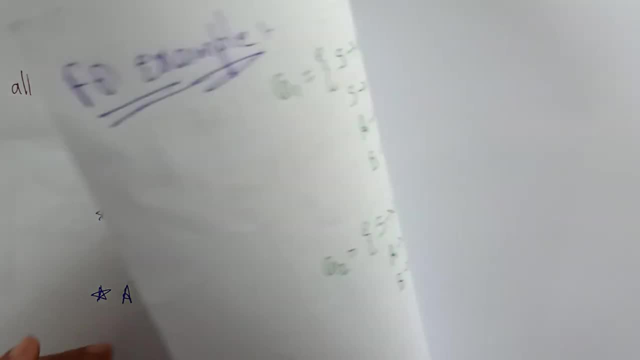 epsilon generating a terminal. So remember these points whenever you are seeing the predictions not starting. it's generating an epsilon and non-terminal is generating two non-terminals or non-terminal is generating a single terminal. So let's see a simple example. whether we have to 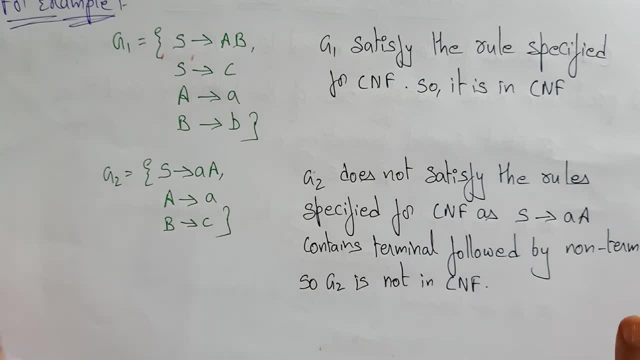 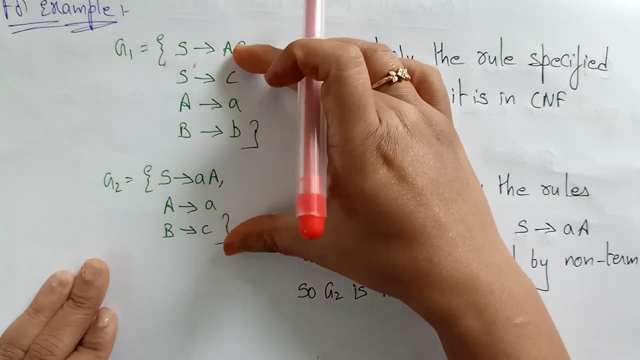 which grammar is in Chomsky normal form and which is not in Chomsky normal form. See here here: S determines AB. This is one context-free grammar. I take in two context-free grammars. in these two context-free grammars I find I need to find out whether these grammar is in Chomsky. 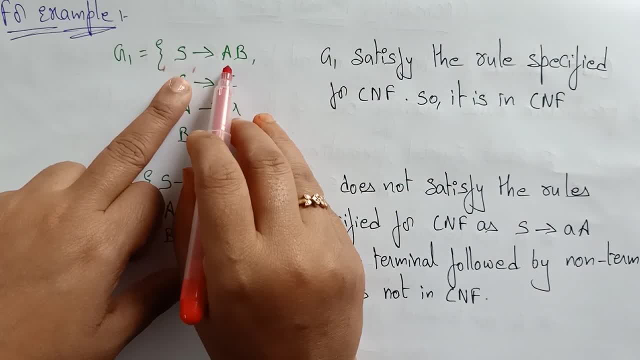 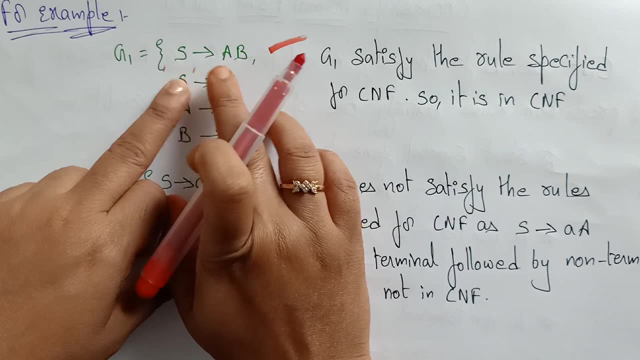 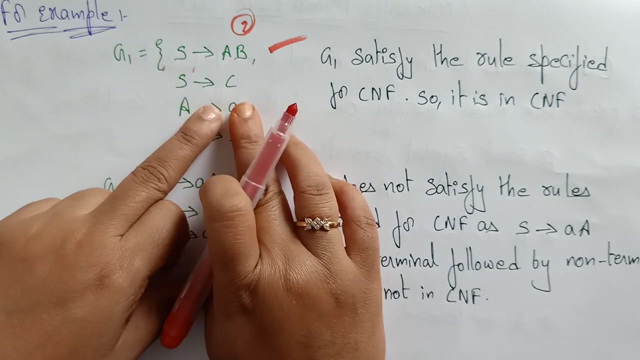 normal form or not? Here S determines AB. Is it following Chomsky normal form? Yes, because a non-terminal has generating two non-terminals. One single non-terminal is generating two non-terminals. that is the second rule. Okay, it is following that. S determines C. Okay, S determines C, which. 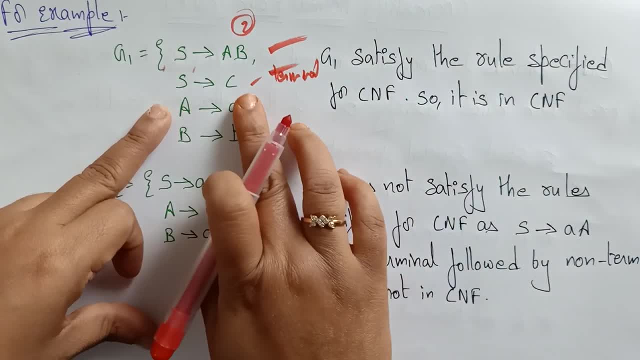 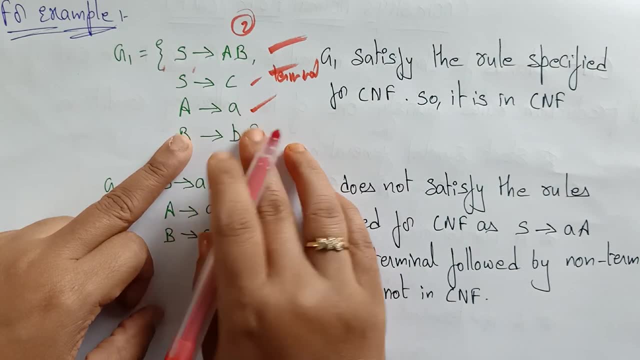 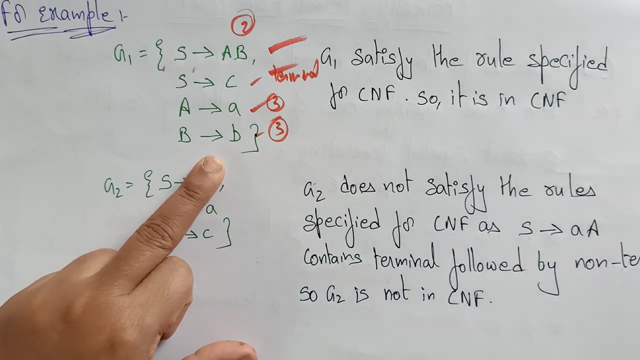 is generating a terminal. So it is in Chomsky normal form and A determines A. Okay, A determines A. This is also Chomsky normal form, but according to the third rule. Okay, according to the third rule, A non-terminal is generating a terminal. That is a third rule. See here A non-terminal. 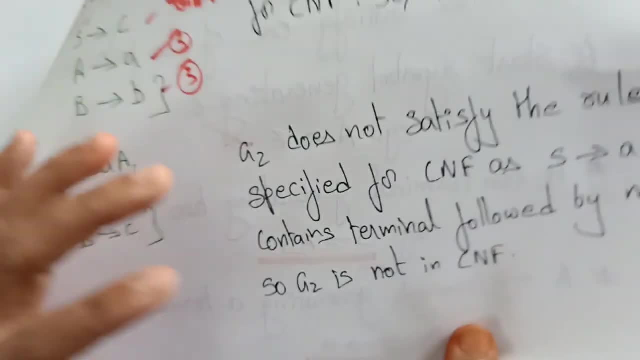 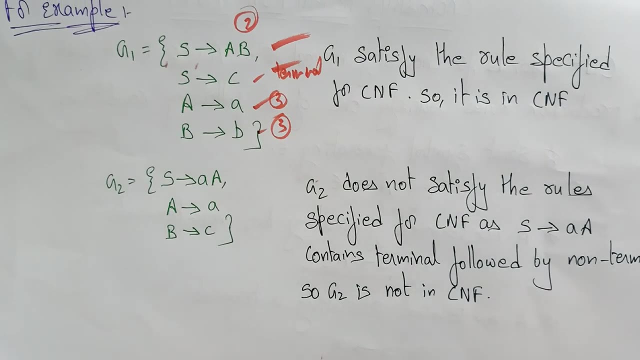 generating a terminal, then you can say that the production is in Chomsky normal form. So either it has to generate an epsilon, or it has to generate a two non-terminals, or it has to generate a single terminal. So here it is. following all each production is following. 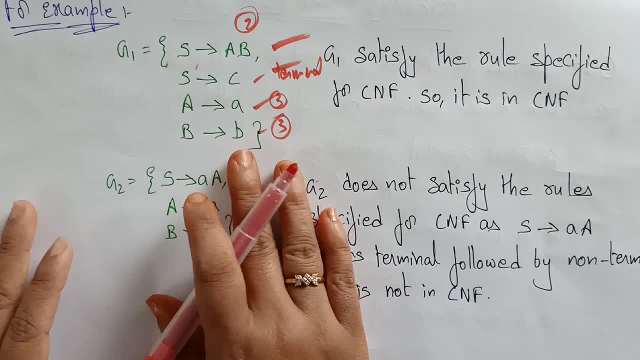 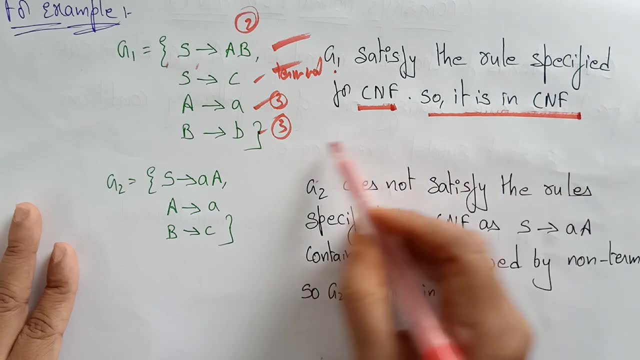 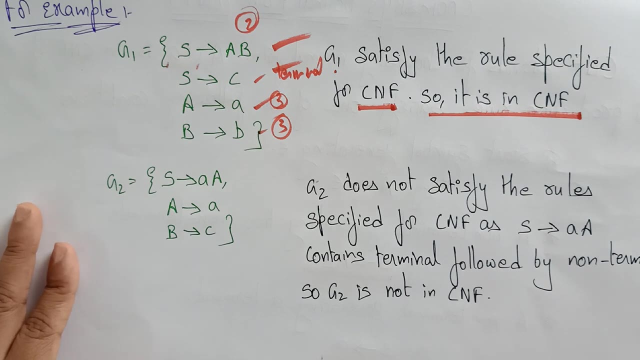 Chomsky normal form production rules. Okay, then you can say: G1 satisfies the rule specified for Chomsky normal form, So it is in CNF. So the given grammar, G1, is in Chomsky normal form. The given context-free grammar, is in CNF by applying the rules. Now let's see these grammar. 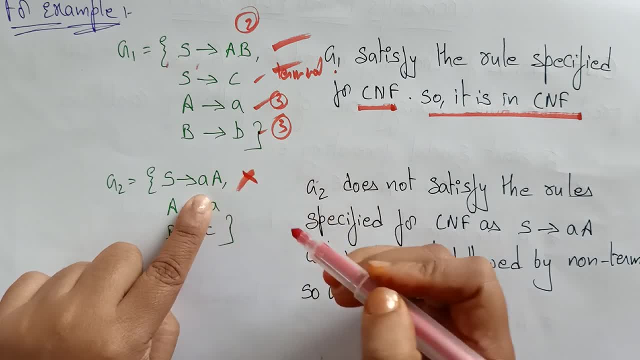 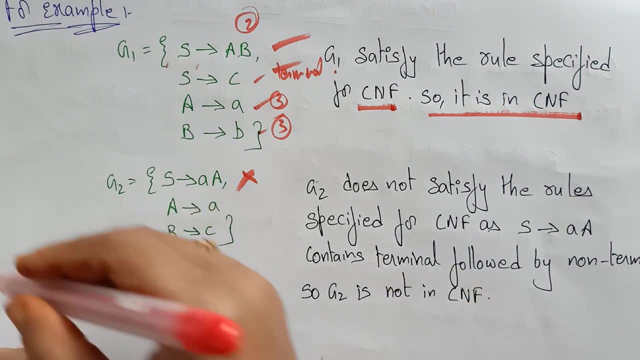 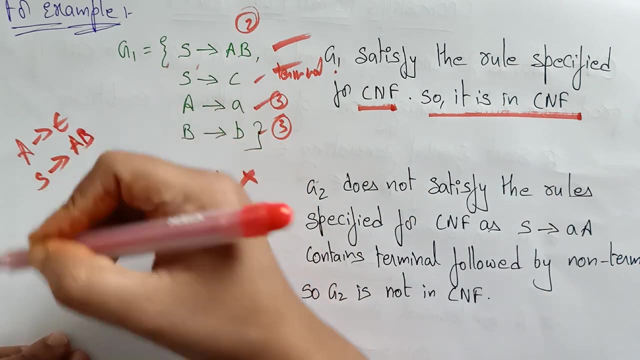 S determines A Is in Chomsky normal form No. How can I say? Because according to our the production, according to our rules, in the Chomsky normal form, either the grammar has to generate an epsilon, either a single non-terminal is generating two non-terminals, either it can a non-terminal is. 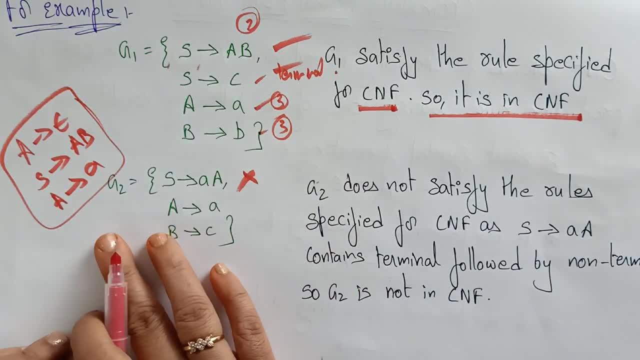 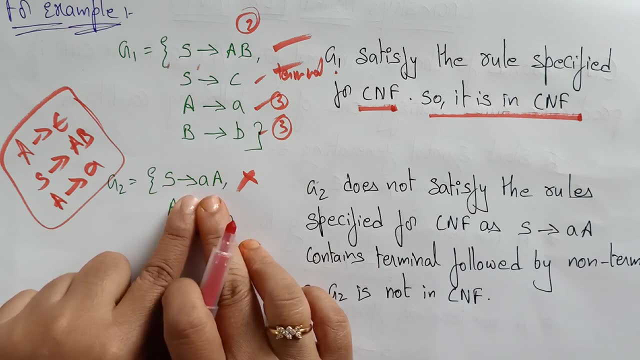 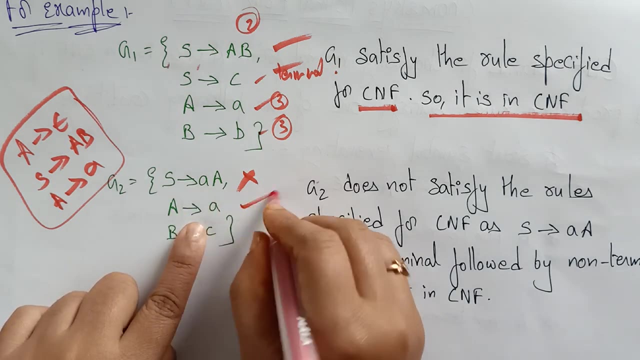 generating a terminal. So these are the three rules that it has to be followed, either any one of this rule, but here it is following. S determines S is generating a non-terminal as well as a non-terminal. Okay, and A determines A. So, okay, this is the. according to the third rule, this will be the. 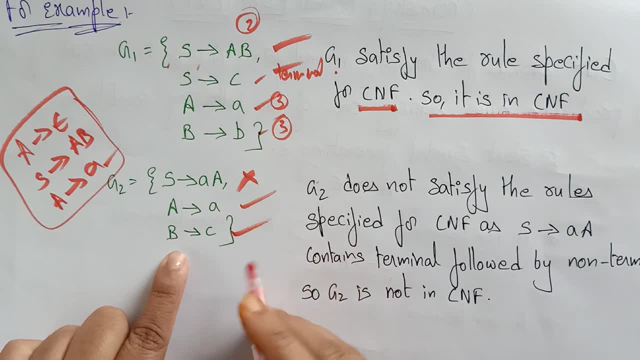 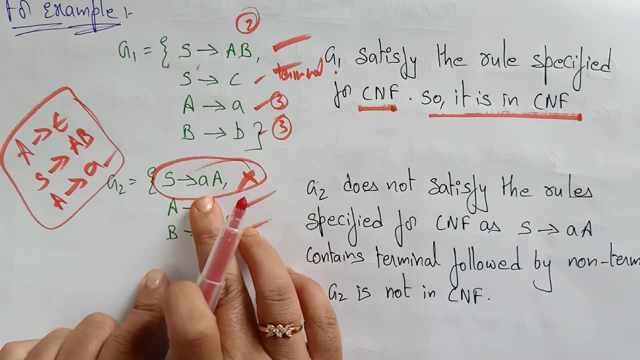 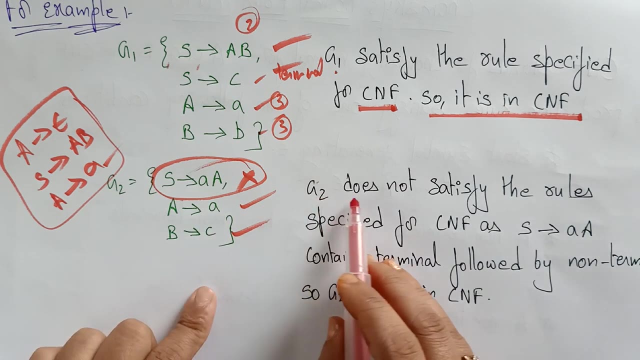 correct. it is in Chomsky normal form and this production is also in CNF. Only this production is not in CNF because this production is following with the terminal. A terminal is followed with a non-terminal which violates the Chomsky normal form rule. So you can say: G2 does not satisfies. 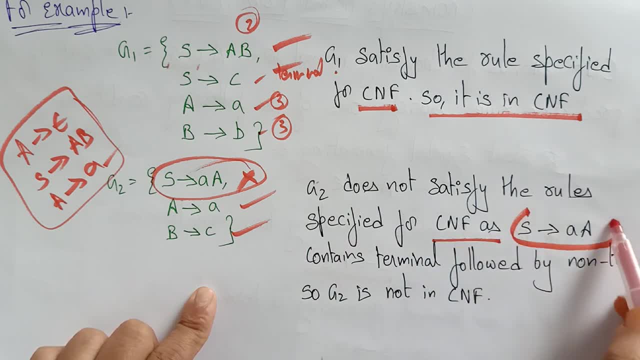 the rule specified for the Chomsky normal form. as S determines, AA A contains a terminal followed by non-terminal, which violates the Chomsky normal form rules. So you can clearly say: G2 is not in CNF. I hope you understand what exactly the Chomsky 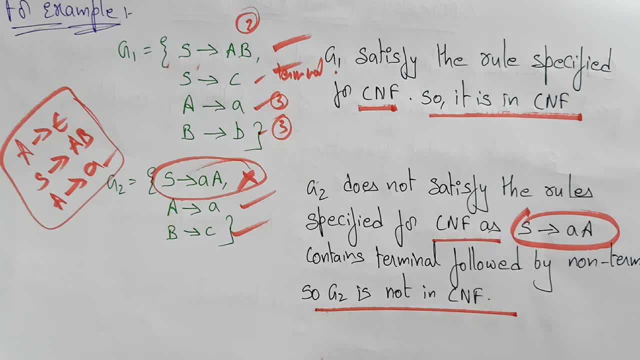 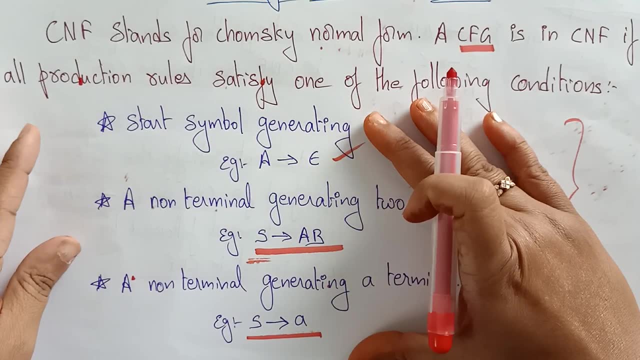 normal form If a given grammar is in, if it is in Chomsky, normal form means it has to follow these rules. So remember these rules, don't forget these rules, because if you know the rules then you can easily identify whether the given grammar is in CNF or not. 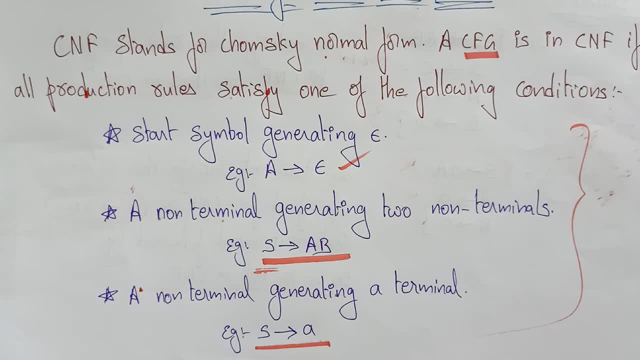 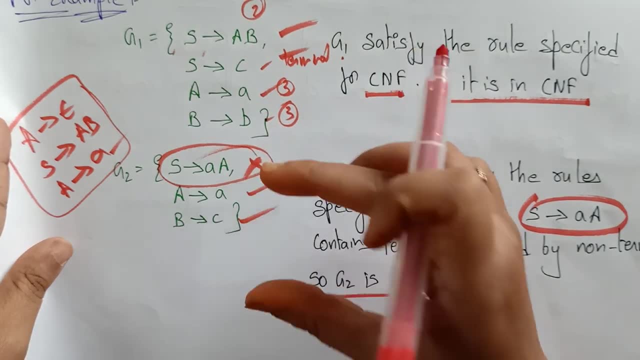 Suppose, if it is not in CNF, we need to convert into CNF. Okay, so here it is not in CNF, If it is not in CNF, it is a context-free grammar only, but it is not in CNF. So how we are going to convert?